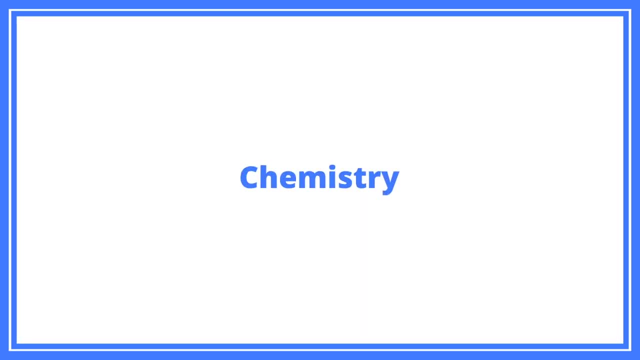 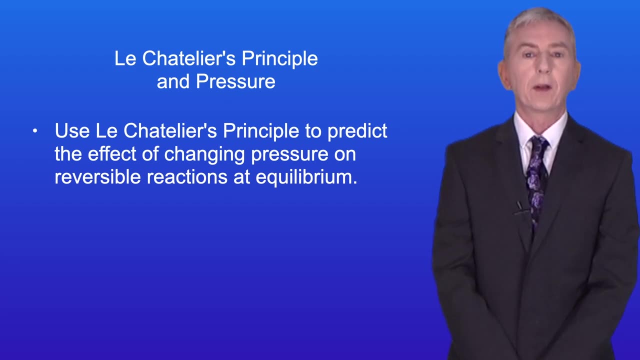 Hi and welcome back to Free Science Lessons. By the end of this video, you should be able to use Le Chatelier's principle to predict the effect of changing pressure on reversible reactions at equilibrium. In the last video we looked at Le Chatelier's principle. Le Chatelier's principle. 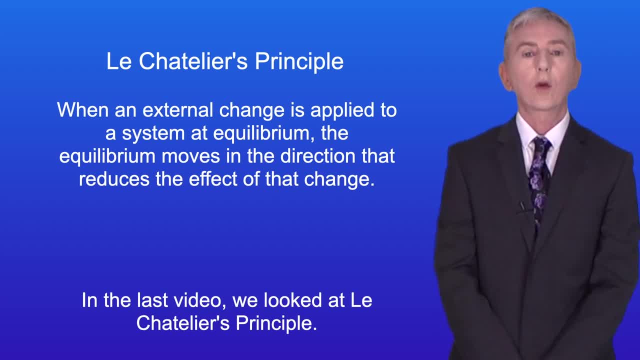 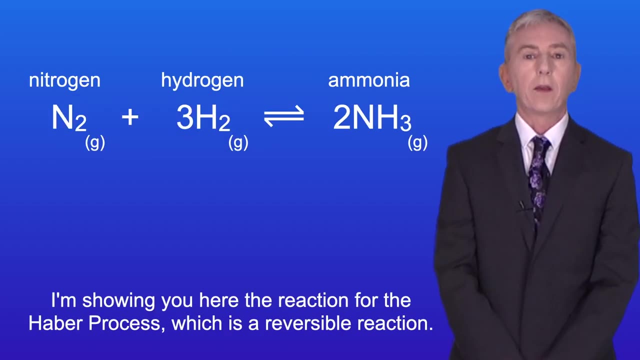 states that when an external change is applied to a system at equilibrium, the equilibrium moves in direction that reduces the effect of that change. In this video we're looking at how Le Chatelier's principle can be applied to reversible reactions involving gases. I'm showing you here the reaction. 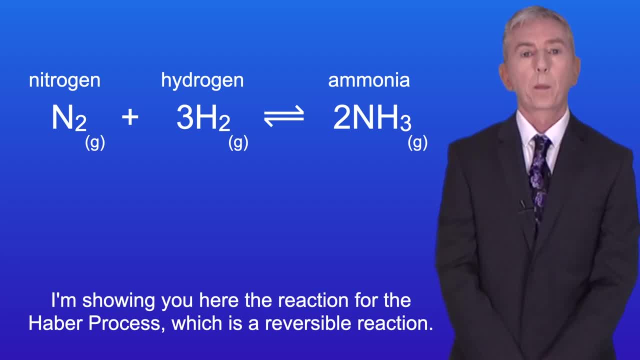 for the Haber process, which is a reversible reaction. In this reaction, the gases nitrogen and hydrogen are reacted to form the gas ammonia. Because this is a reversible reaction, the ammonia can also convert back to nitrogen and hydrogen. With reactions involving gases, we can change the position of the equilibrium by changing the 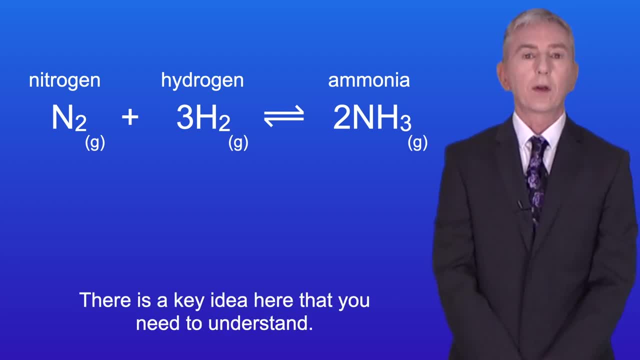 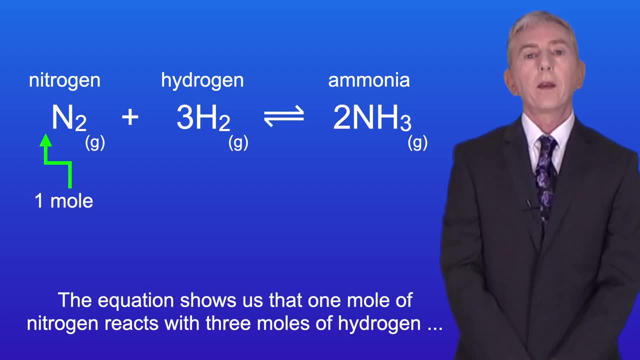 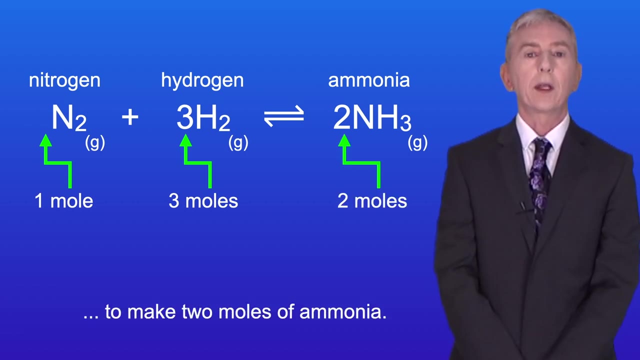 pressure. Now there's a key idea here that you need to understand: Gas pressure is proportional to the number of moles of gas present. The equation shows us that one mole of nitrogen reacts with three moles of hydrogen to make two moles of ammonia. We have a total of four moles. on the 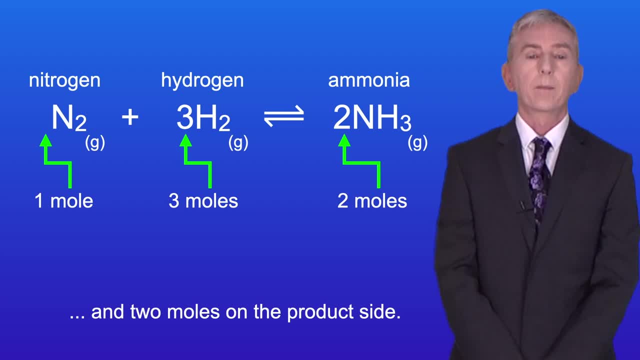 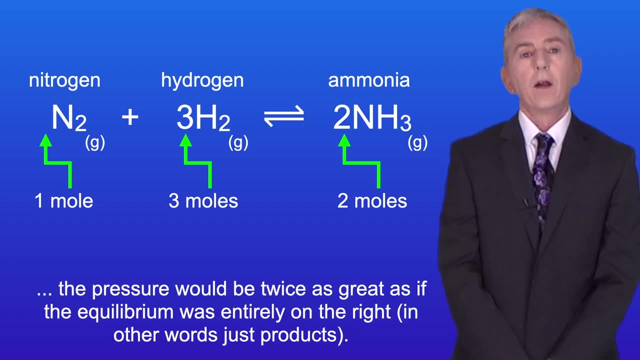 reactant side and two moles on the reaction side. So we have a total of four moles on the reactant side and two moles on the reaction side. So what that means is that if the equilibrium was entirely on the left, in other words, just reactants, the pressure would be twice as great as if the equilibrium was entirely on the right, in other words, just products. 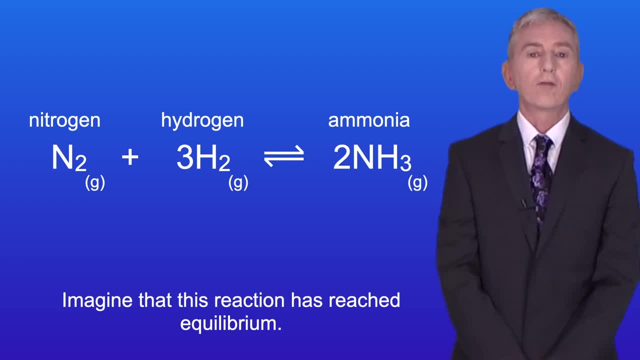 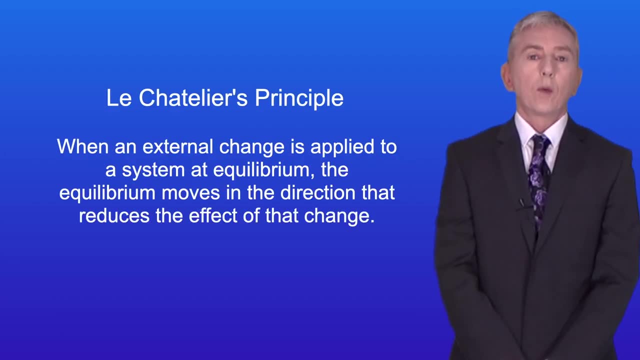 Okay, so imagine that this reaction has reached equilibrium. What would happen to the position of the equilibrium if we increase the pressure? Well, going back to Le Chatelier's principle, we know that when an external change is made to the equilibrium, the pressure will increase. Well, going back to Le Chatelier's principle, we know that when an external change is made to the equilibrium, the pressure will increase. So any new change applied to a system at equilibrium, the equilibrium moves in the direction that reduces the effect of that change. 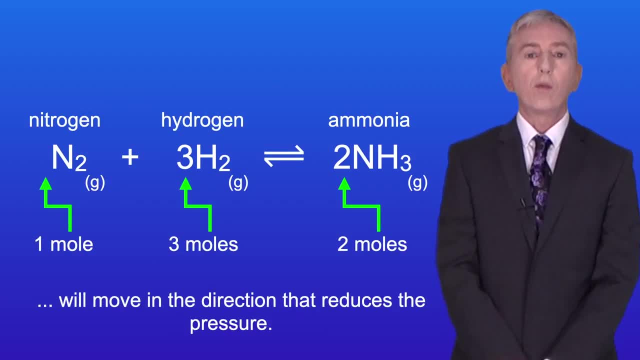 We're increasing the pressure, so this means that the equilibrium will move in the direction that reduces the pressure. As we've seen, the right-hand side of the equation has fewer moles than the left-hand side, So that means that, in order to reduce the pressure, the equilibrium will move toward.